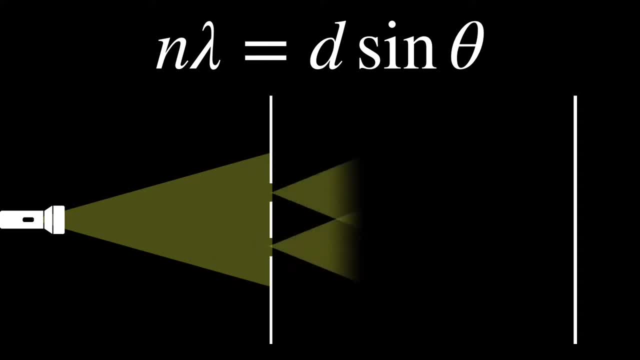 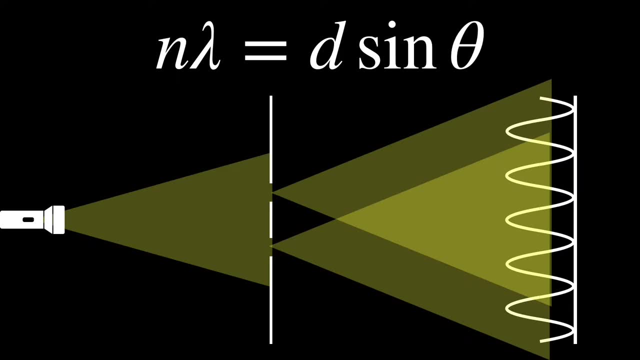 of the same amplitude goes through two slits. The light diffracts through both of those slits and then interferes with itself on the other side of the slits. This has been shown experimentally to produce a pattern on a screen in which the intensity of the light oscillates from zero to 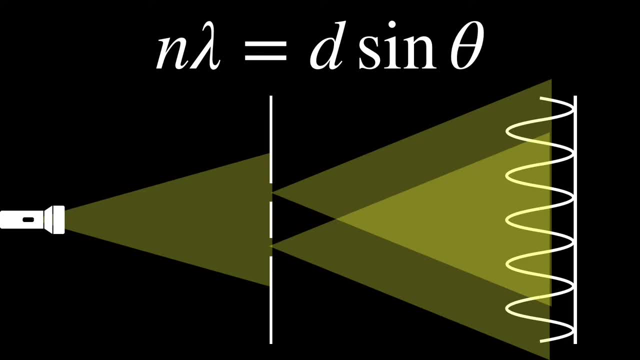 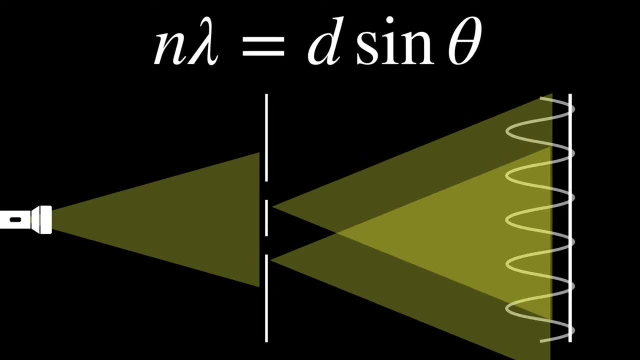 some maximum, which is the graph I'm showing in the diagram. So how can this be explained theoretically? It begins by simplifying the situation. We don't need to focus on all of the light at once, but just the beams that happen to land on the same spot on the screen. 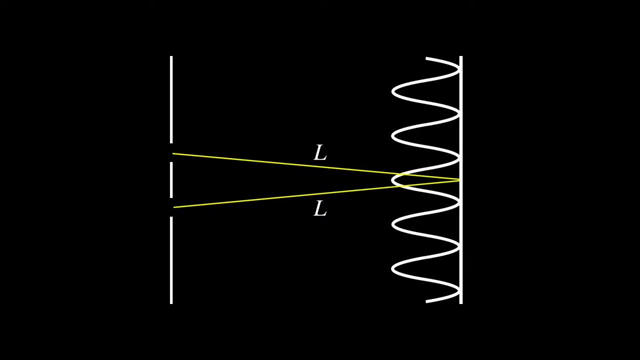 Let's first consider two beams of light that travel to the center of the screen. From the symmetry of the situation, maybe you can see that the distance between that the two beams travel is exactly the same, Since the light had a constant phase difference initially. 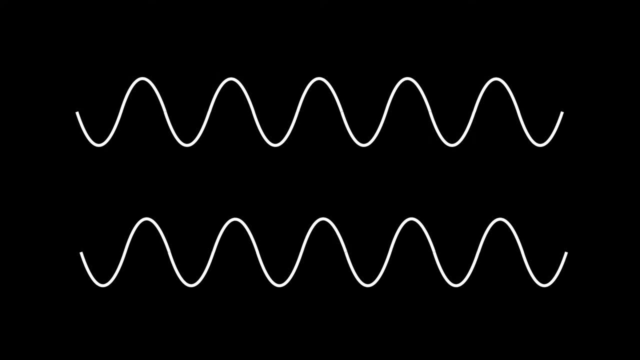 we can leverage the principle of superposition to see that the waves will constructively interfere, since they're perfectly lined up. Hence it is quite clear that the center of the screen should be a maximum, so we'll be able to label that n equals zero, because it's essentially a trivial. 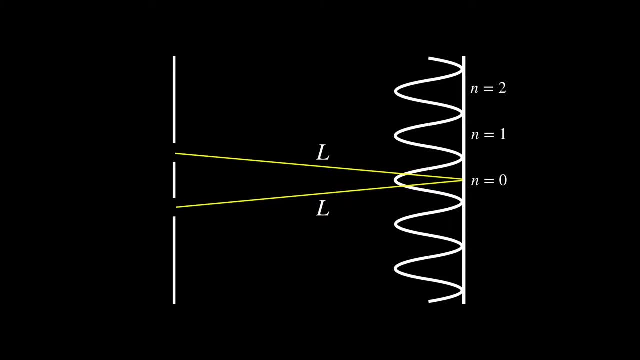 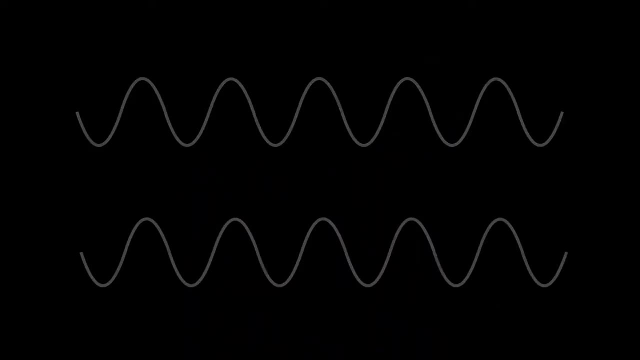 maximum and, as you'll see in a moment, that's helpful for the derivation as well. Now let's consider how the first maximum, n equals one, is possible. In order for constructive interference to occur, the waves have to be in phase, The troughs and the peaks have to line up right. But that can happen. 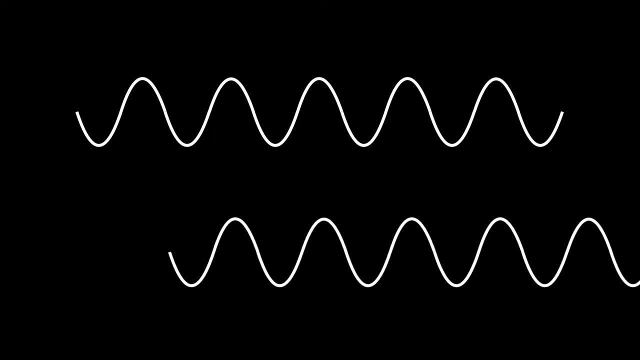 even if the other wave travels a full wavelength longer. In fact, the waves would be in phase, even if the other traveled two or three or four wavelengths longer. As you can hopefully see in the diagram, the peaks and the troughs totally line up, even when there's this path. difference of 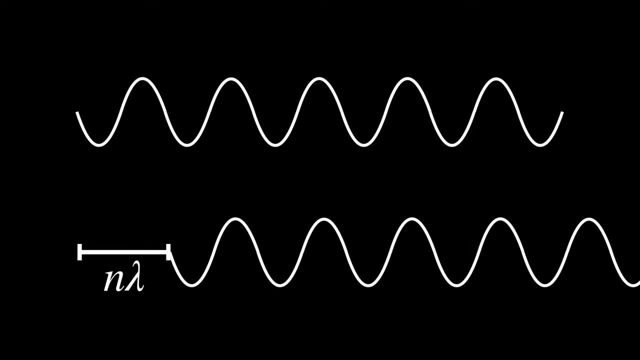 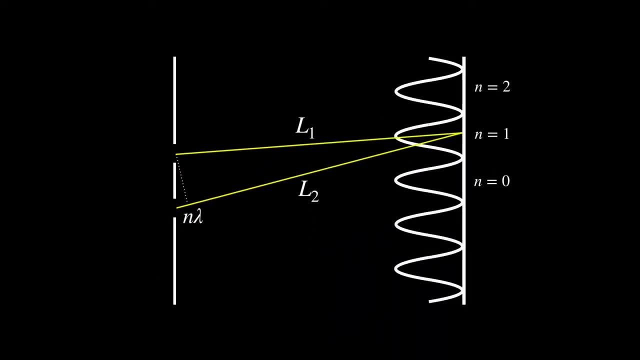 one wavelength. In general, if the path difference is an integer number of wavelengths, constructive interference occurs. Returning to our diagram, that means that L2 must be an integer number of wavelengths longer than L1.. In this case it's just one wavelength longer, but I'm trying to. 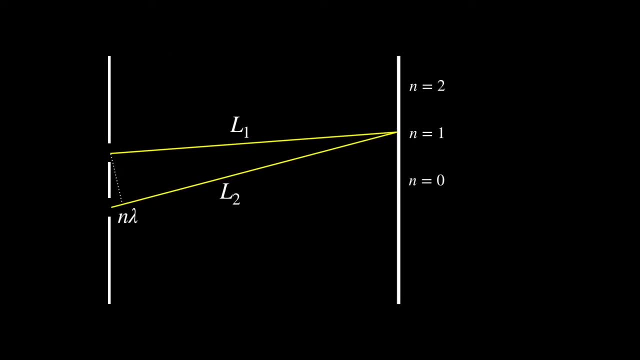 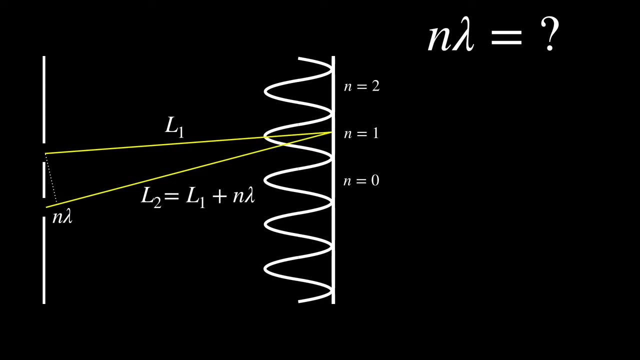 keep this as general as possible to apply to all maximums. so we're going to keep it as n lambda. So now the question becomes: how do we know when the path difference will be an integer number of wavelengths? Unfortunately, this is where we need to make some use of the geometry of the situation. 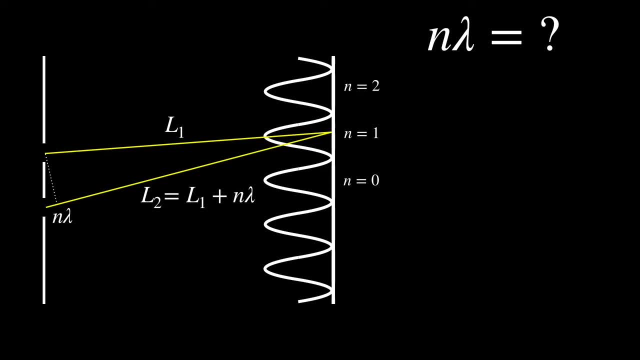 and some valid approximations. Often the approximations are the hardest part to understand, so we'll work on making those clear. OK, to find the relationship, we'll want to only use things that are available to use on this diagram and kind of in the experiment. So let's add two lines and 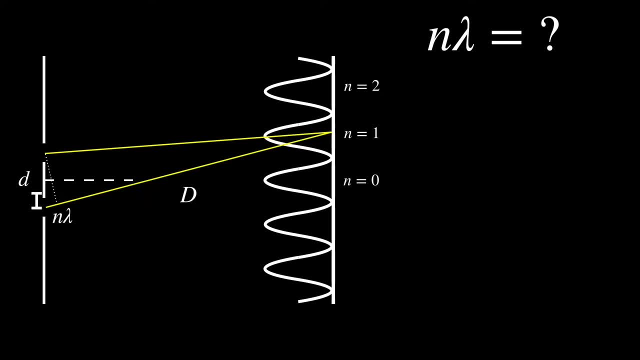 assign them variables. Let lowercase d be the distance between the slits and capital D be the distance from the slits to the screen. Finally, I'll add a line from the center of the slits to the maximum. Now it's important to realize that this diagram is absolutely not to scale. 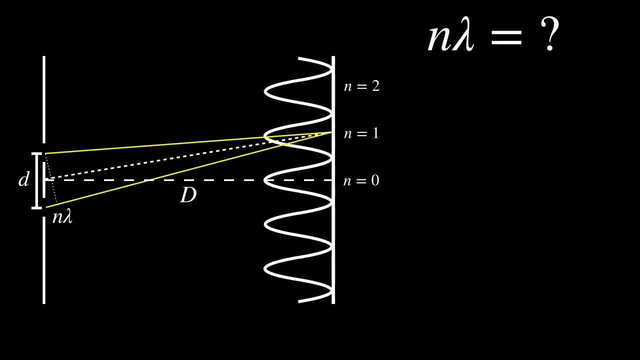 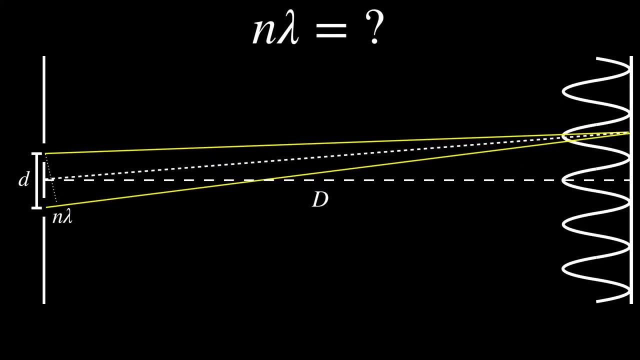 Capital D will be much, much larger than lowercase d. In any experiment you do normally, capital D would be hundreds of times longer than lowercase d. So maybe you can see that if capital D is really much, much larger than lowercase d, then the two lines, the horizontal lines and the 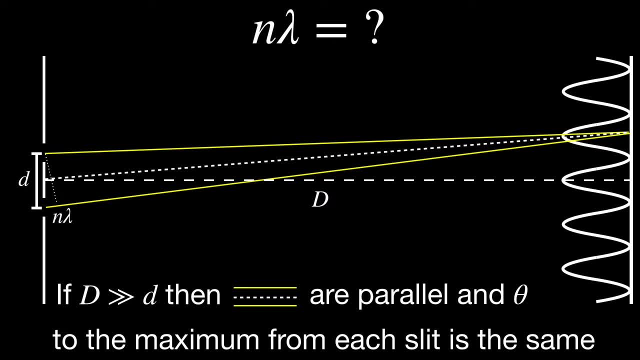 beams of light and the line from the center of the slits to the maximum will essentially be parallel, because they're at such tiny angles to each other in order to meet after capital D meters. Honestly, you could treat all three lines as starting and ending on the same point. 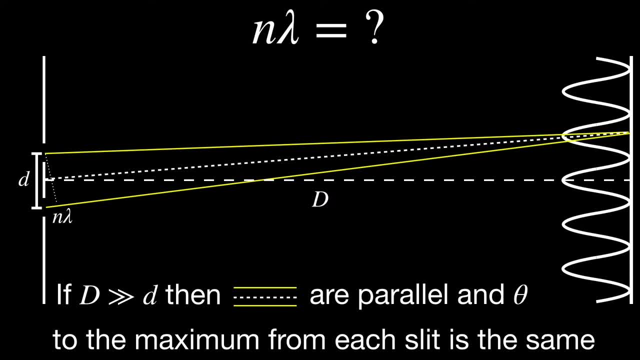 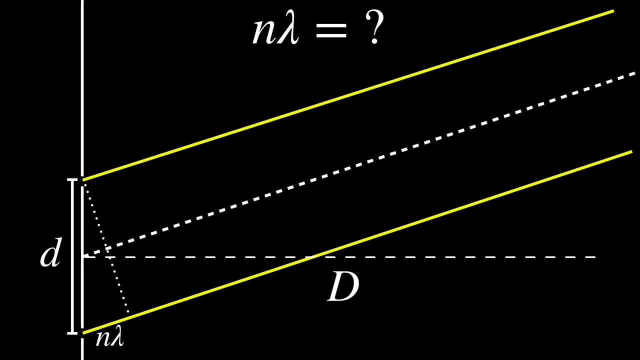 Not only are they parallel, but when you're zoomed out like this, for all intents and purposes they're the same line. But to exaggerate the distance between them and show how parallel they are, let's look closer. We can then add an angle theta between capital D and the line from the. 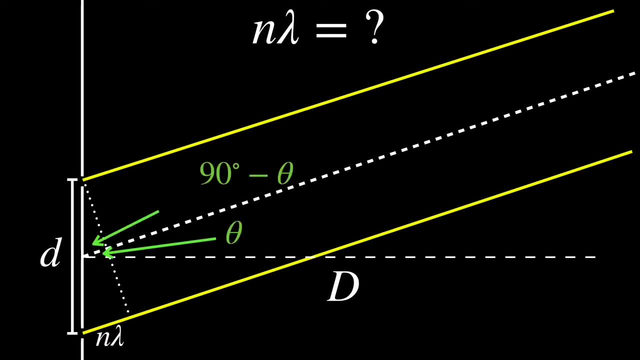 slits to the maximum, Then this angle is 90 minus theta, since capital D is perpendicular to lower lowercase d, And then, because this is a right triangle, this angle is theta. After that, using a bit of right angle trigonometry, with lowercase d as the hypotenuse and n lambda as 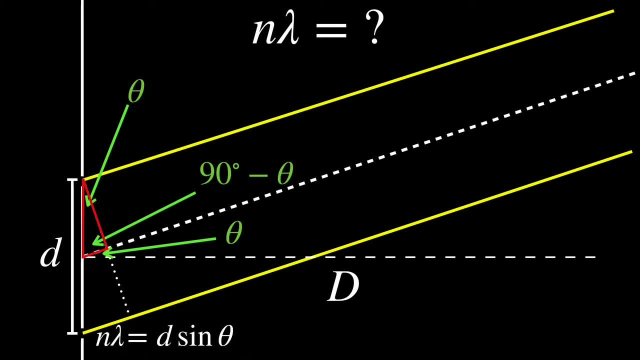 the opposite. we know that n lambda equals d sine theta, Which is one of the formulas you can use. Then we can take this formula and apply a little more math to find the fringe spacing in units of meters. All we have to do is add the variable s for the